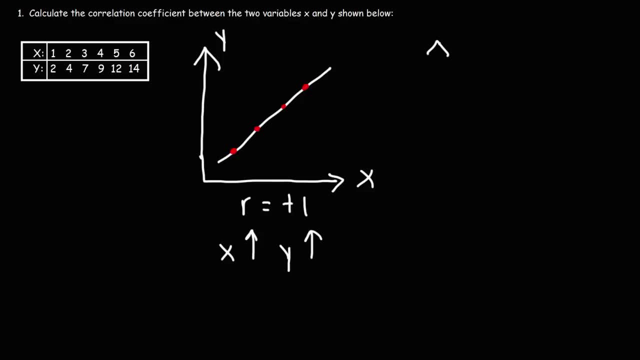 direct relationship between x and y. Now here's another scenario. Here we have points on the line, but notice, the line is going down, And so the correlation coefficient will be equal to negative one As x increases, y decreases, And so in that case we have an inverse relationship. 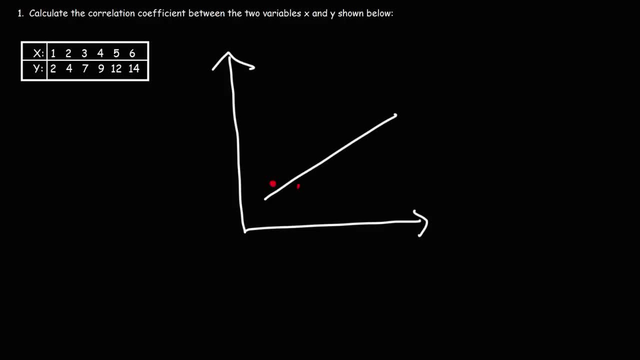 Now, in this example, the points are not necessarily on the line, but they're close to it, And so these points, they have somewhat of a linear relationship, but not exactly one. So in this case, r is going to be somewhere between zero and one. It's positive because 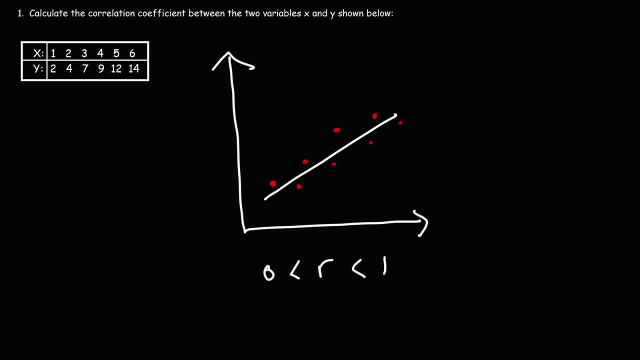 this line is increasing. It has a positive slope, but it's not exactly one. If we were to put a number to it, it might be 0.8 or something, Whereas let's say, if you have a similar line, but let's say the points are more scattered about that line, 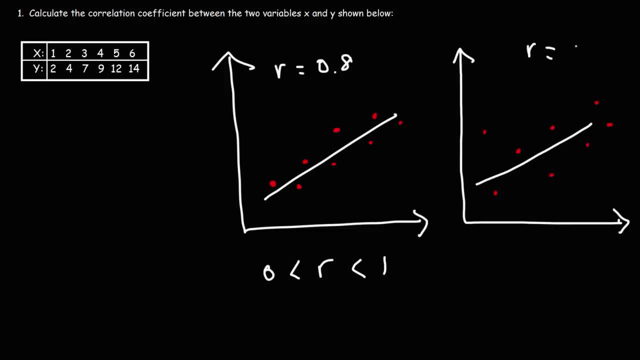 the r value will be less. It might be 0.7 or 0.6.. It could be completely different, but it's somewhere between zero and one. But the point is this though: The closer that the points are next to the line, r is going to be closer to one These points, they're further. 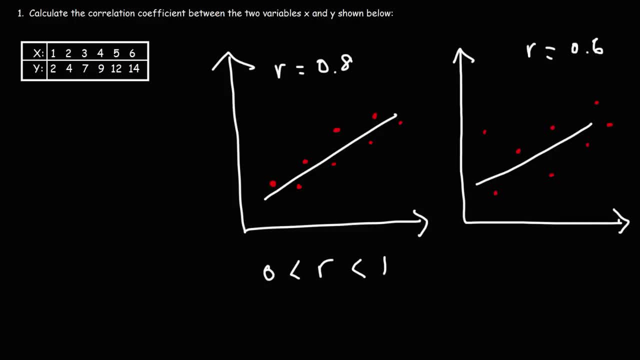 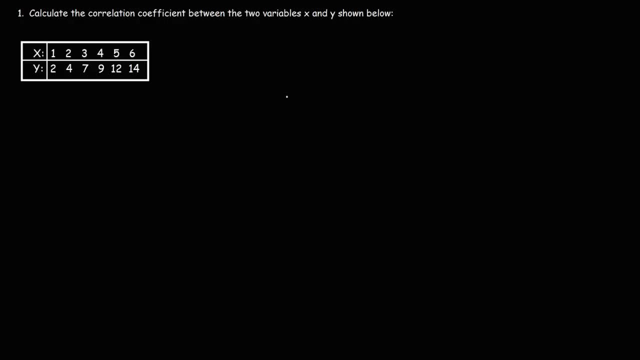 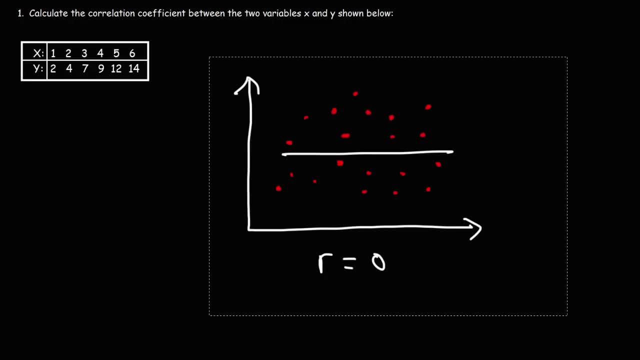 apparent correlation. So the correlation co-efficient. coefficient really tells us the strength of the linear relationship between two variables. If these two variables have no linear relationship, r is going to be close to 0.. If there is a strong linear relationship, r is going to be close to. 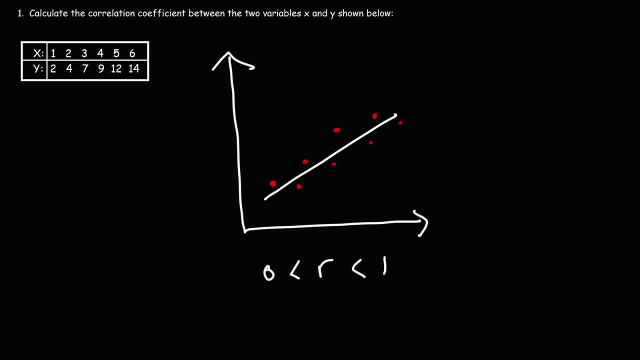 this line is increasing. It has a positive slope, but it's not exactly one. If we were to put a number to it, it might be 0.8 or something, Whereas let's say, if you have a similar line, but let's say the points are more scattered about that line, 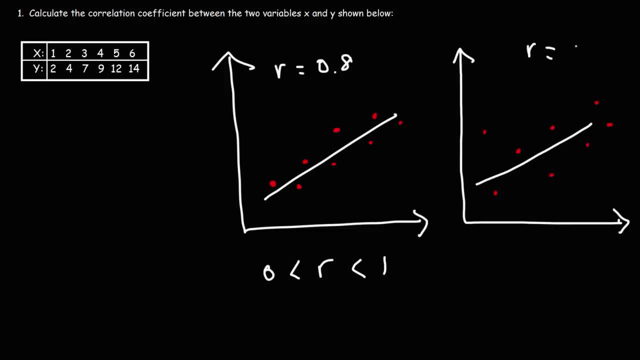 the r value will be less. It might be 0.7 or 0.6.. It could be completely different, but it's somewhere between zero and one. But the point is this though: The closer that the points are next to the line, r is going to be closer to one These points, they're further. 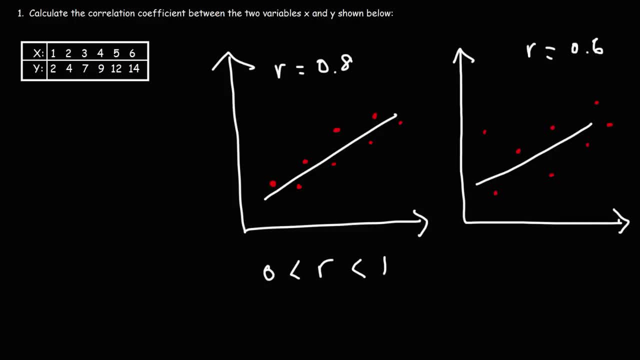 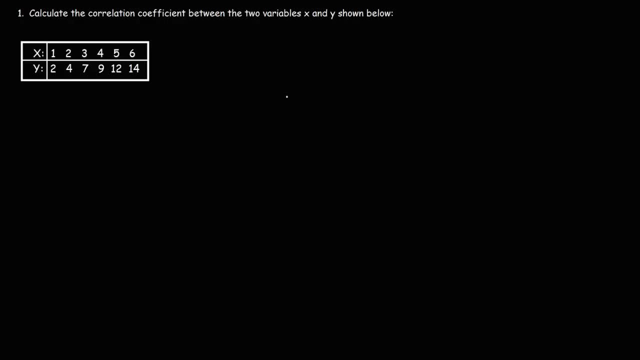 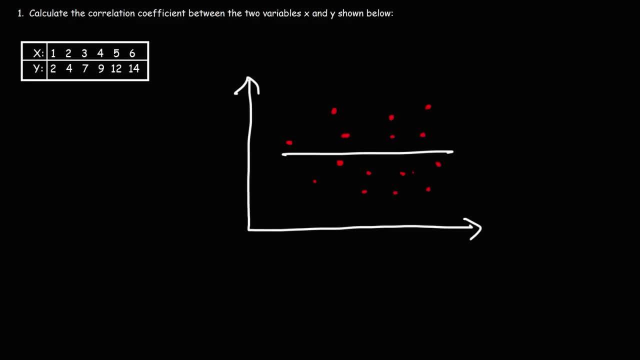 everywhere. In this case, r could be very close to zero for a situation like that where there's no apparent correlation. So the correlation co-efficient 0.4.. 0.4.. coefficient really tells us the strength of the linear relationship between two variables. 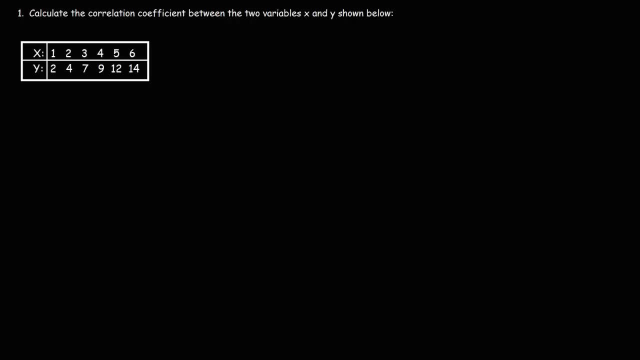 If these two variables have no linear relationship, r is going to be close to zero. If there is a strong linear relationship, r is going to be close to either positive one or negative one, depending on the slope of the line. Now let's take a minute and calculate. 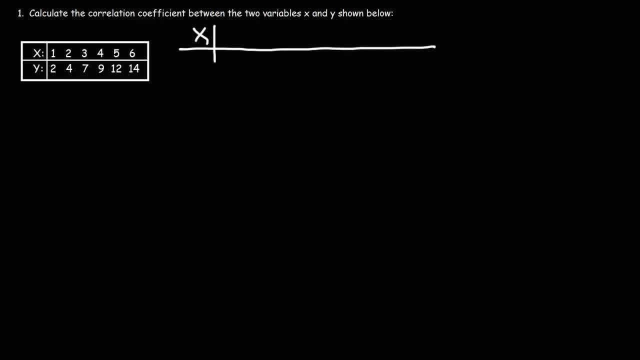 the correlation coefficient. So we're going to make a table containing the columns x, y, and then the product of x, y, and then x squared, followed by y squared. So for x we have the numbers 1,, 2,, 3,. 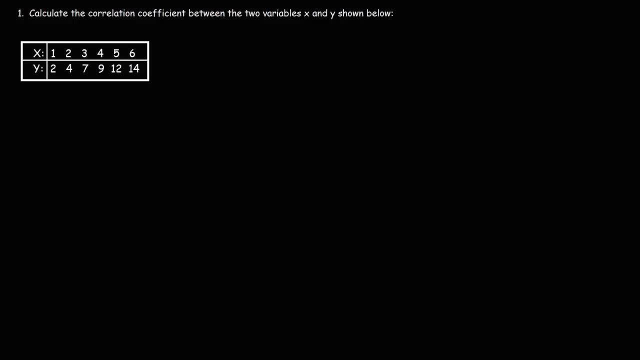 either positive 1 or negative 1, depending on the slope of the line. Now let's take a minute and calculate the correlation coefficient. So we're going to make a table containing the columns x, y, and then the product of X, Y, and then 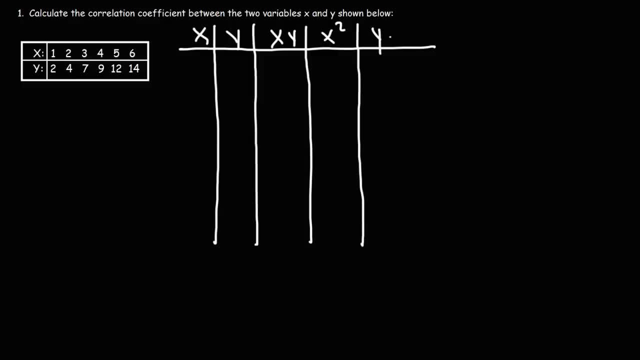 x squared, followed by y squared. So for x, we have the numbers 1, 2, 3, 6, 7, 8, 9, 10, 11, 11, 12, 13, 12, 13, 15, 22, 23, 23, 23, 24, 25, 26, 25, 27, 28, 29, 60. I'm going to make a table containing the columns x, y, and then the product of XY, and then the products of x, y, and then x squared, followed by y squared. so for x, we have the numbers one, two, three. 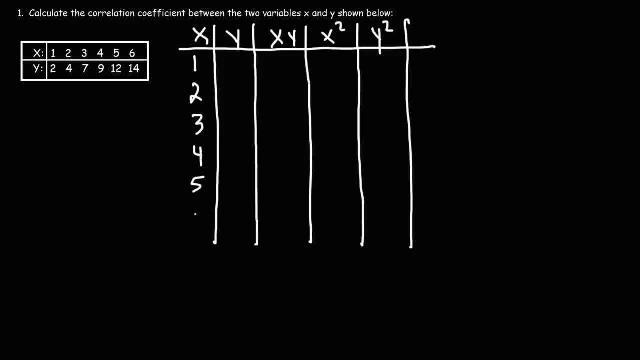 So for x we have the numbers one, two, three, three, four, five and six. So let's extend this a bit. Alright, now let's fill in this table. So next let's put the y values, which are two, four, seven, nine, twelve, fourteen. 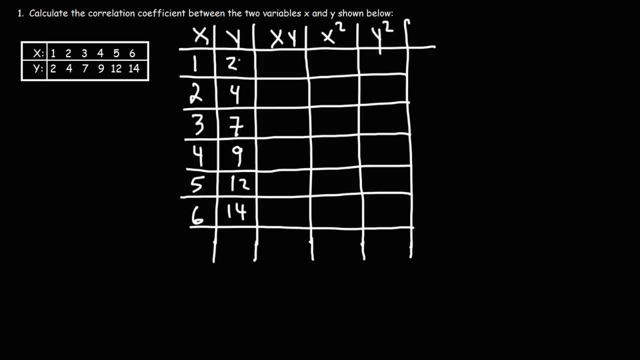 Moving on to the next column, we need to multiply x and y, So one times two, that's going to be two, And then, if we multiply two and four, we're going to get eight. Next, we're going to multiply three and seven, which is twenty-one. 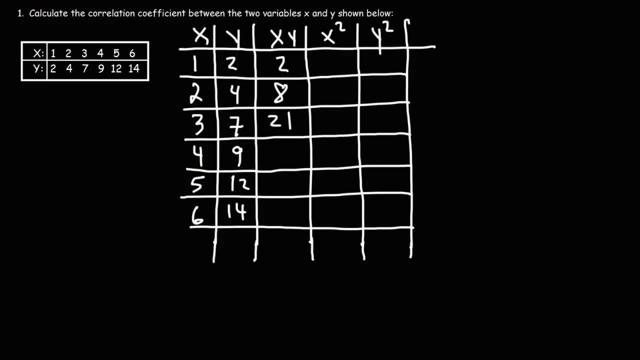 And then four times nine, that's thirty-six. Five times twelve is sixty, And then six times fourteen. Six times ten is sixty. Six times four is twenty-four. When you add sixty and twenty-four, that gives you eighty-four. Now moving on to the next, column x, squared. 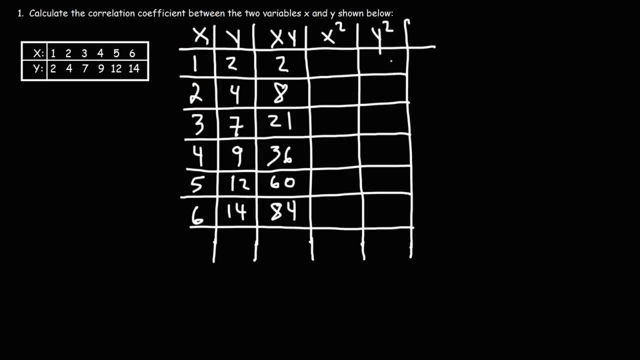 So we're going to square the values that we see in the x column. One squared is one, Two squared is one. Two squared is four. Three squared is nine. Four squared is sixteen. Five squared is twenty-five. Six squared is thirty-six. 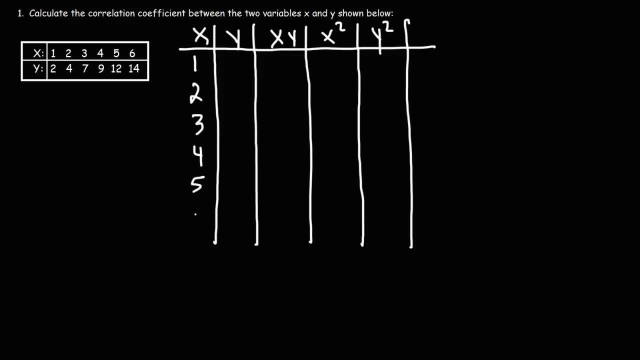 4,, 5, and 6.. So let's extend this a bit. All right, now let's fill in this table. So next let's put the y values, which are 2,, 4,, 7,, 9,, 12,, 14.. 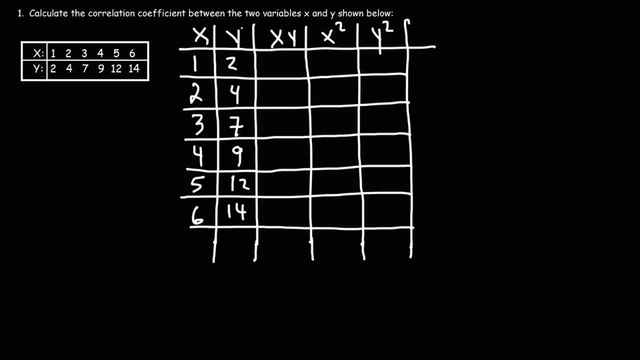 Moving on to the next column, we need to multiply x and y. So 1 times 2, that's going to be 2.. And then, if we multiply 2 and 4, we're going to get 8.. Next, we're going to multiply x and y. 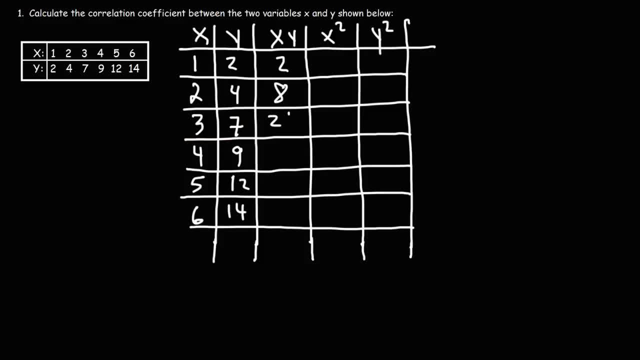 So we're going to multiply 3 and 7,, which is 21.. And then 4 times 9,, that's 36.. 5 times 12 is 60. And then 6 times 14.. 6 times 10 is 60.. 6 times 4 is 24.. 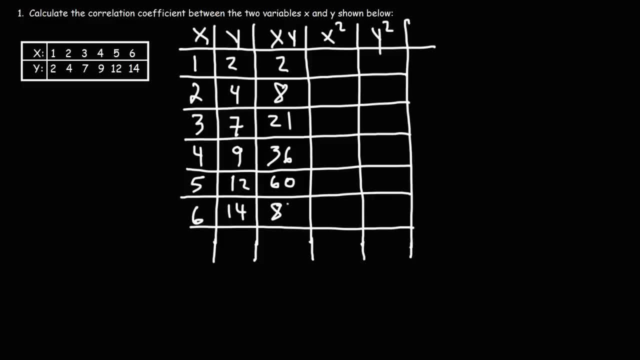 When you add 60 and 24, that gives you 84.. Now, moving on to the next column, x squared. So we're going to square the values That we see in the x column: 1 squared is 1.. 2 squared is 4.. 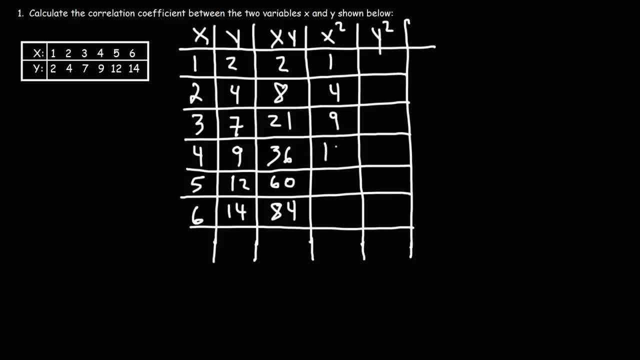 3 squared is 9.. 4 squared is 16.. 5 squared is 25.. 6 squared is 36.. Now for y squared. all we're going to do is square the values in the y column. So 2 squared is 4.. 4 squared is 16.. 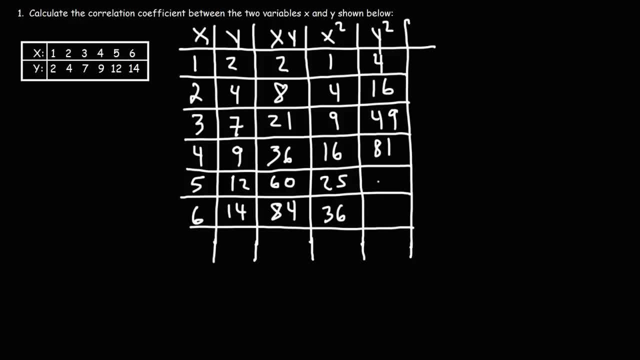 7 squared is 49.. 9 squared is 81.. 12 squared is 14.. 44. And 14 squared is 196.. Now our next step is to sum up each column. So if we take the sum of the x values, 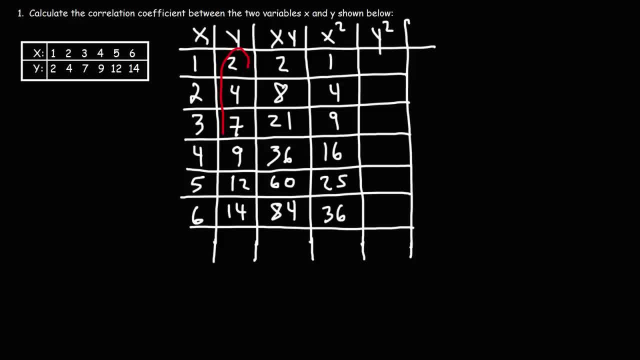 Now for y squared. all we're going to do is square the values in the y column. So two squared is four, Four squared is sixteen, Seven squared is forty-nine, Nine squared is eighty-one, Twelve squared is one, forty-four And fourteen squared is one, ninety-six. 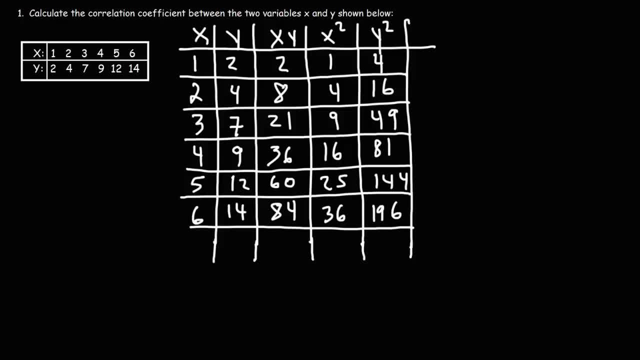 Now our next step is to sum up each column. So if we take the sum of the x values, it's going to be one plus two plus three, plus four plus five plus six, That's going to be twenty-one. Let me put this in a different color. 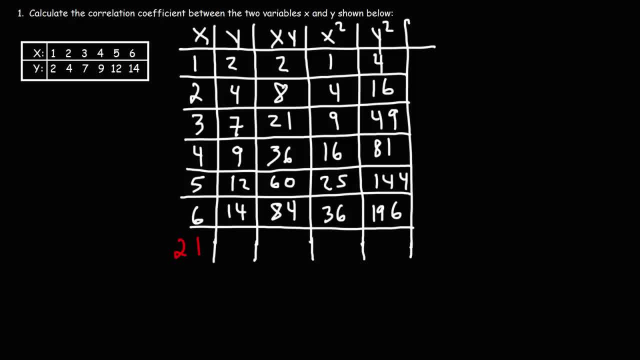 Now let's take the sum of the y values: Two plus four plus seven plus nine plus twelve plus fourteen, So that gives us a sum of forty-eight. Now we need to determine the sum of the product of x and y. So two plus eight plus twenty-one plus thirty-six plus sixty plus eighty-four. 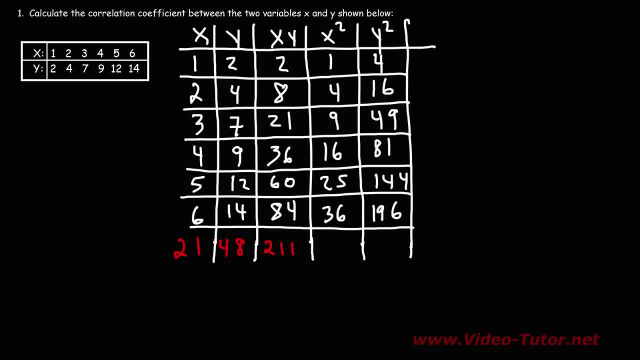 So that's going to give us two, eleven. Now the sum of the x squared values one plus four plus nine plus sixteen plus twenty-five plus thirty-six, So that's going to be ninety-one. And then the sum of the y squared values four plus sixteen plus twenty-five plus thirty-six. 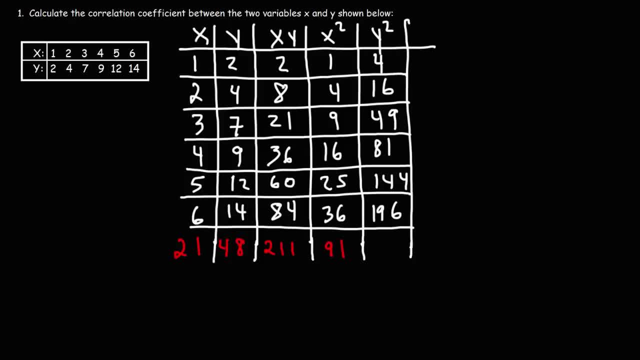 So that's going to be ninety-one, Forty-nine, eighty-one, one, forty-four, and then plus one is one, ninety-six. So that's going to be four, ninety. So this is the sum of the x values. Forty-eight is the sum of the y values. 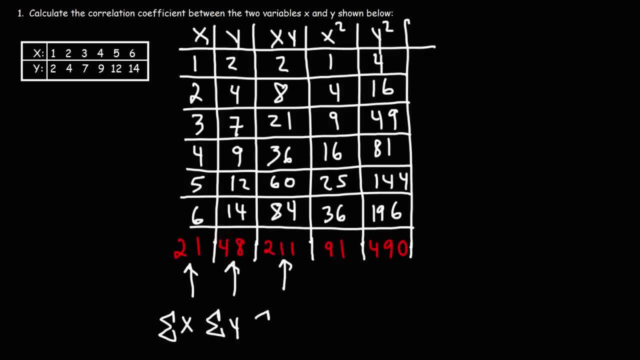 And two, eleven, that's the sum of x, y, X squared, and four, ninety is the sum of y squared. So once we have those numbers in red, we can now plug in the information into the formula to get the answer we need. 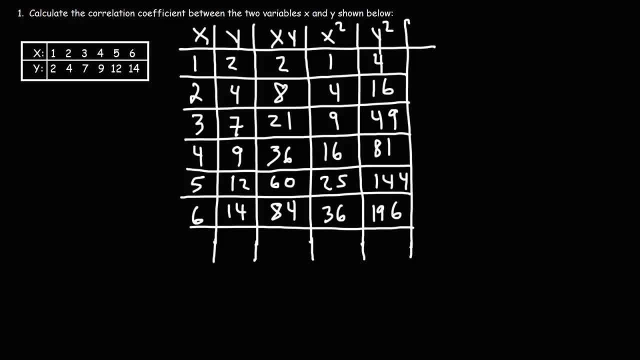 it's going to be 1 plus 2 plus 3 plus 4 plus 5 plus 6.. That's going to be 21.. Let me put this in a different color. Now let's take the sum of the y values. 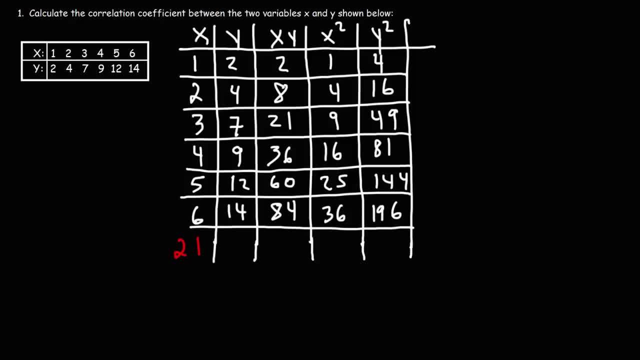 2 plus 4 plus 7 plus 9 plus 12 plus 14.. So that gives us a sum of 48.. Now we need to determine the sum of the product of x and y, So 2 plus 8 plus 21, plus 36 plus 60 plus 84.. 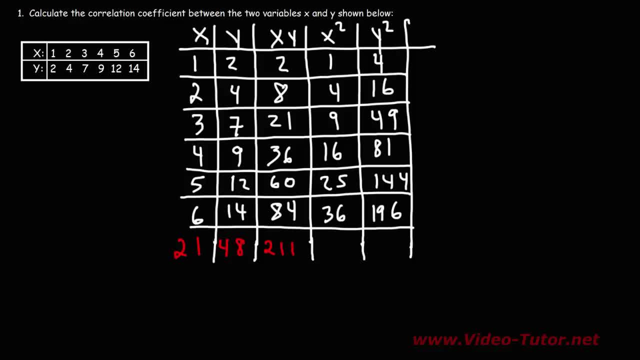 So that's going to give us 211.. Now the sum of the x squared values: 1 plus 4 plus 9 plus 16 plus 25 plus 36.. So that's going to be 91.. And then the sum of the x squared values: 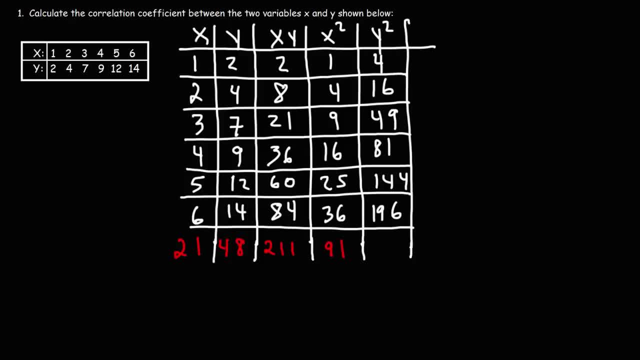 4 plus 16.. 49,, 81,, 144, and then plus 196.. So that's going to be 490.. So this is the sum of the x values, 48 is the sum of the y values And 211, that's the sum of x- y. 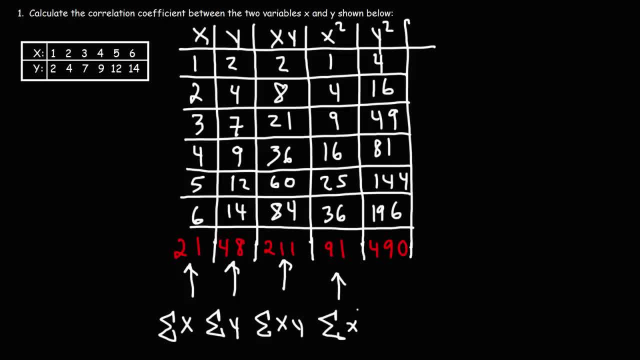 91 is the sum of x squared And 490 is the sum of y squared. So once we have those numbers in red, we can now plug in the information into the formula to get the answer we need. So I'm going to delete everything up to there. 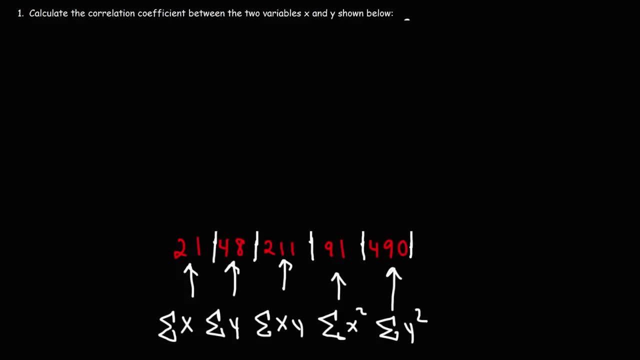 And here's the formula that we need. So the correlation coefficient r, which in some equations is represented by the Greek symbol rho. It's equal to n times the sum of x, y minus the sum of x times the sum of y Divided by the square root. 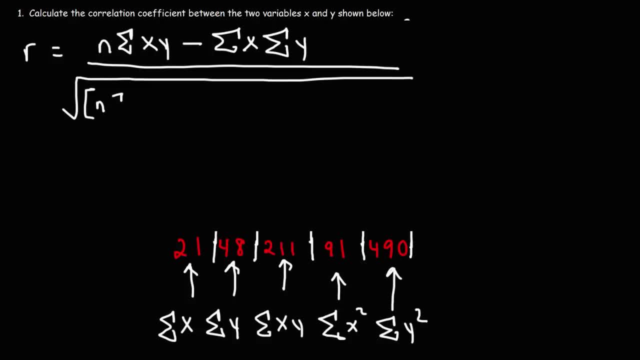 And inside the square root it's going to be n times the sum of the x squared values minus the sum of x values, But we're going to square that, So be careful with that difference. And then it's going to be n times the sum of the y squared values minus the sum of the y values, and then squared. 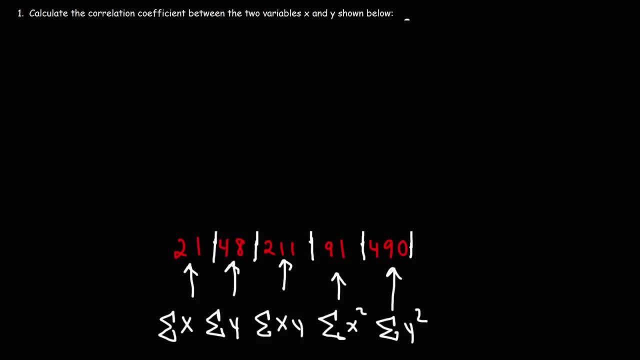 So I'm going to delete everything up to there, And here's the formula that we need. So the correlation coefficient r, which in some equations is represented by the Greek symbol rho, It's equal to n. Okay, It's equal to n times the sum of x, y minus the sum of x times the sum of y divided by. 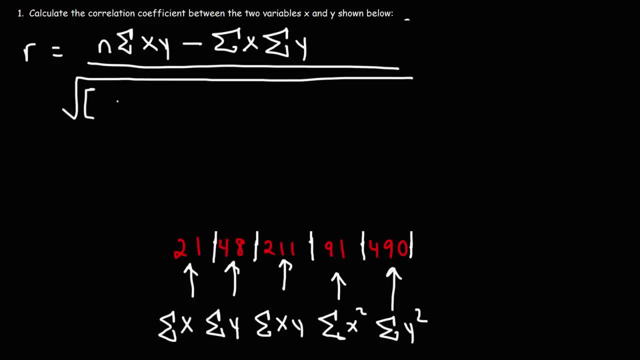 the square root And inside the square root it's going to be n times the sum of the x squared values minus the sum of x values, but we're going to square that, So be careful with that difference. Then it's going to be n times the sum of the y squared values minus the sum of the y values. 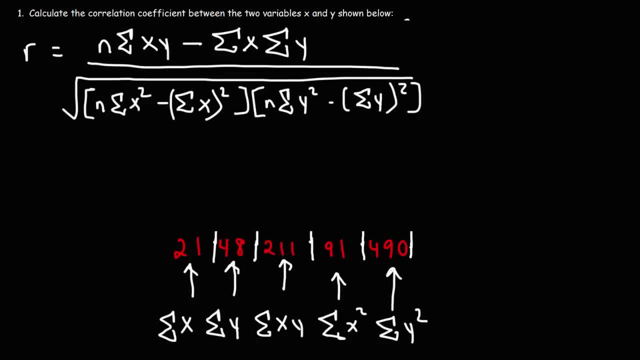 and then squared. So let's plug in everything into that formula. So it's going to be n. well, we need to know what n is And, if you recall, there were six x values: One, two, three, four, five, six. 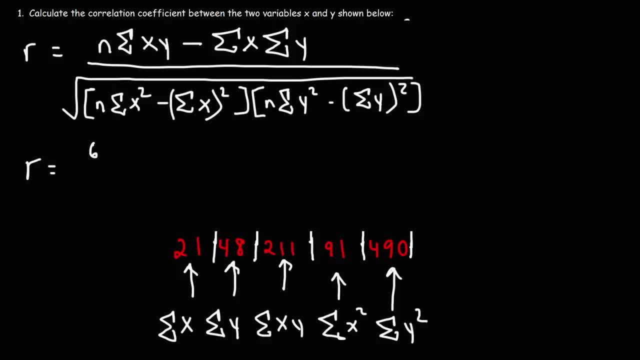 So n is the number of x, So n is the number of values that we have in one single column, So that's six in this example, And then times the sum of x- y, which is 211 minus the sum of the x values. 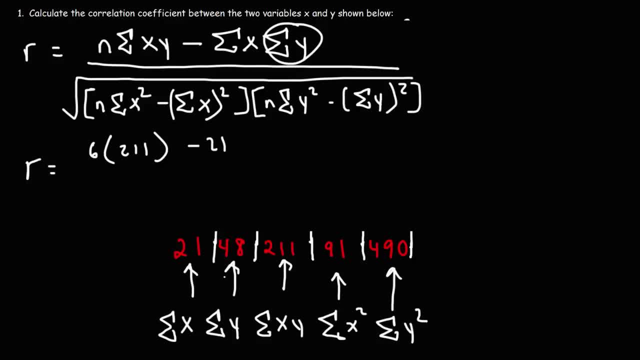 So that's 21.. And then the sum of the y values, that's 48.. So at this point we just got to plug everything into this formula, And then it's going to be n times the sum of the x squared values, which is 91 minus. 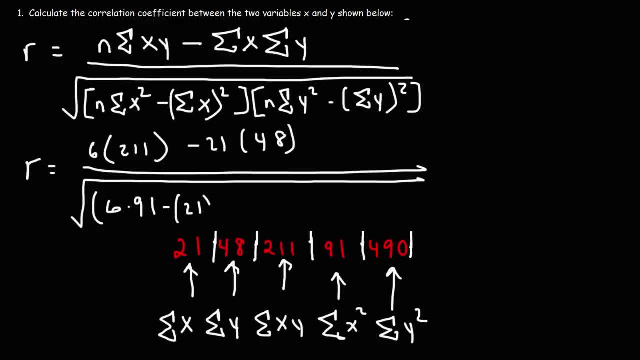 the sum of the x values squared. So that's 21 squared. Then it's going to be n times the sum of the y squared values, which is 490.. I sped that up a little. Let's type it in, OK. 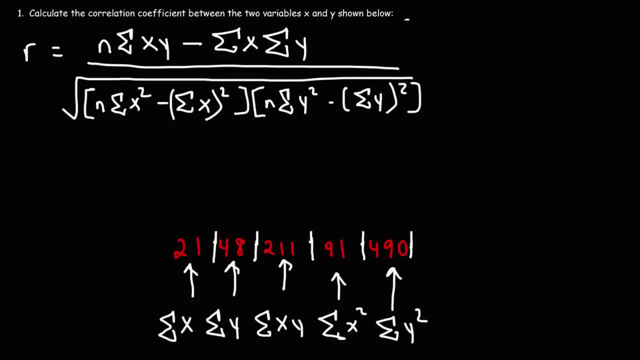 So let's plug in everything into that formula. So it's going to be n. Well, we need to know what n is And, if you recall, there were six x values: One, two, three, four, five, six. 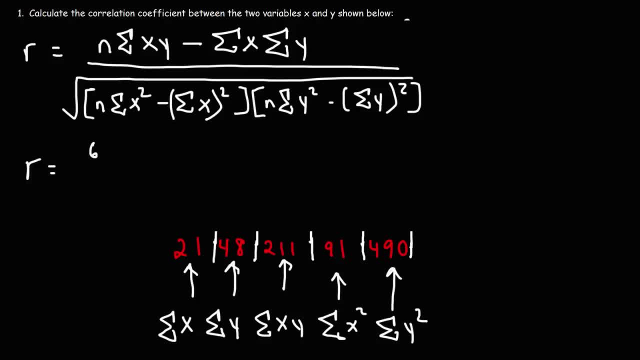 So n is the number of values that we have in one single column, So that's six in this example, And then times the sum of x- y, which is 211 minus the sum of the x values, So that's 21.. 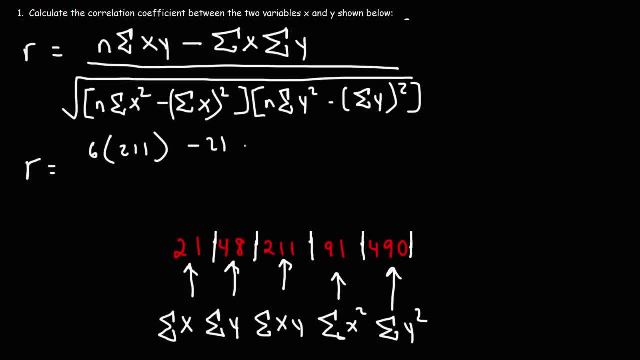 And then the sum of the y values, That's 48.. So at this point we just got to plug everything into this formula, And then it's going to be n times the sum of the x squared values, which is 91 minus the sum of the x values squared. 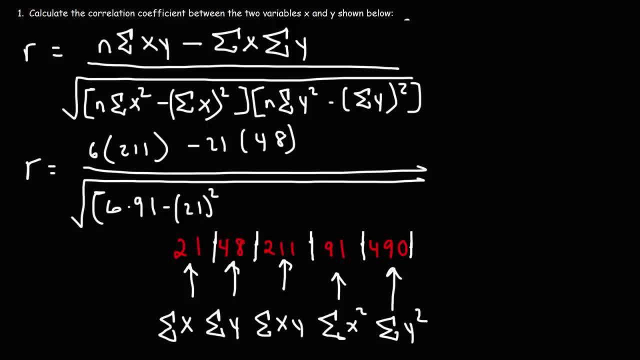 So that's 21 squared. Then it's going to be n times The sum of the y squared values, which is 490.. And then minus the sum of y, which is 48, but squared. So that's what we have so far in this example. 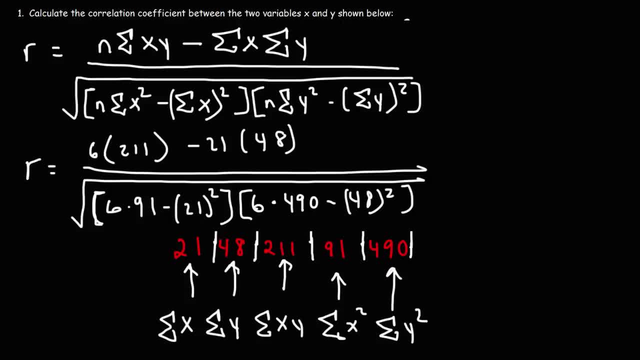 Now let's plug everything in So we can get rid of these numbers. Six times 211 is 1266.. And 21 times 48, that's 1008.. Now, six times 91, that is 546.. 21 squared is 441.. 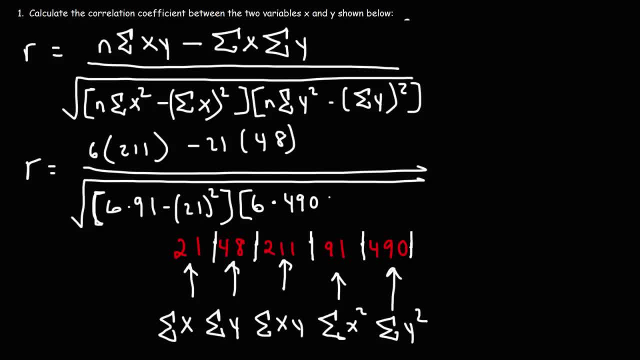 That isolate, That's lost, And then minus the sum of y, which is 48, but squared. So that's what we have so far in this example. Now let's plug everything in So we can get rid of these numbers. 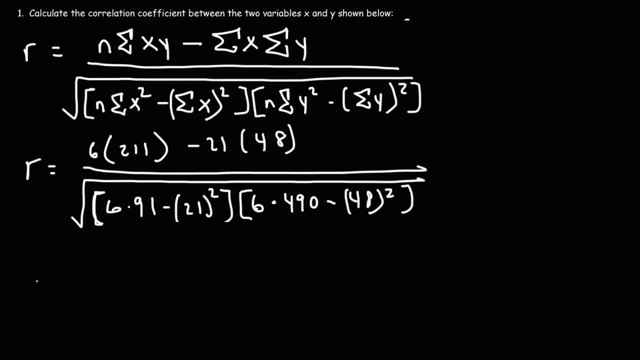 6 times 211 is 1266.. And 21 times 48,, that's 1008.. Now 6 times 91,, that is 545.. 21 squared is 441.. Now, 6 times 490 is 2940.. 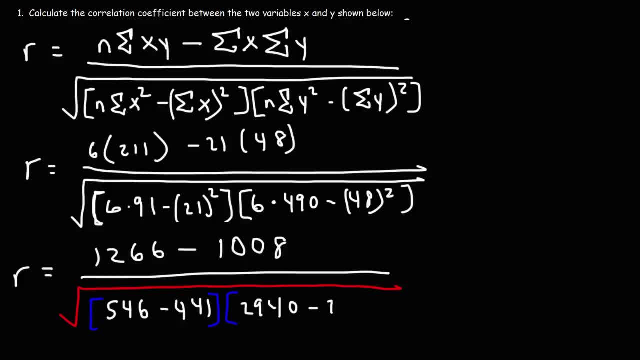 And then 48 squared, that's 2304.. Now let's subtract 1266 by 1008.. So that's 258.. And then we have 546 minus 441, which is 105.. And then 2940 minus 2304, that's 636.. 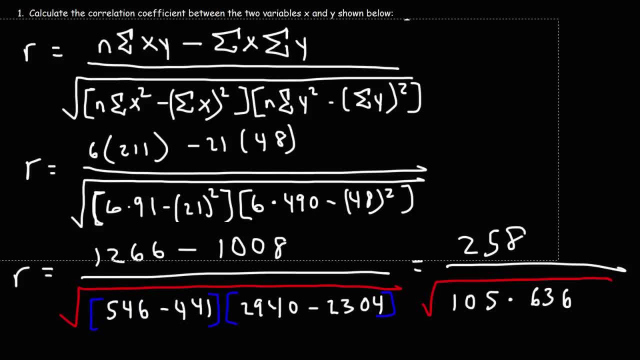 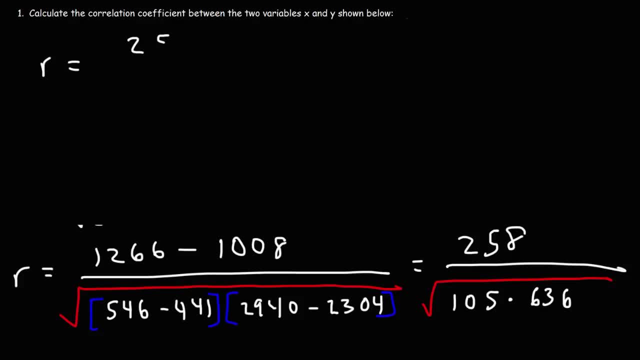 636.. So far we have: R is equal to 258, divided by the square root. And now let's multiply those two numbers, So 105 times 636, that's 66,780.. So if we take 258 and divide it by the square root of 66,780,, 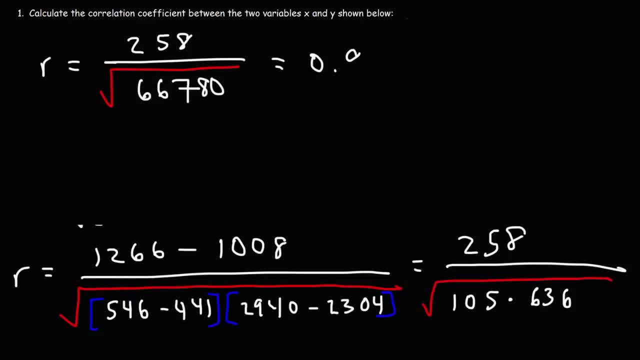 we get an R value of 0.998.. So this R value is very high. This indicates that there is a very strong linear relationship between the X and Y variables that we have in this problem, And the fact that it's positive tells us that the slope is positive.